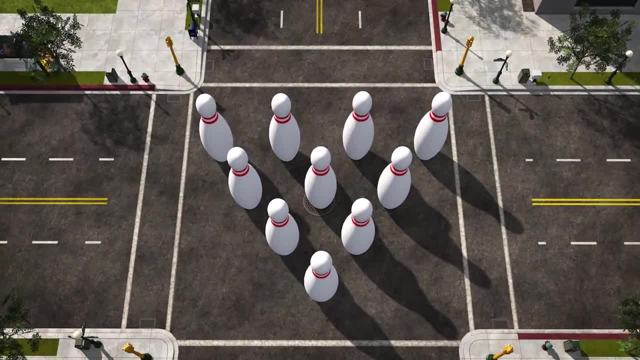 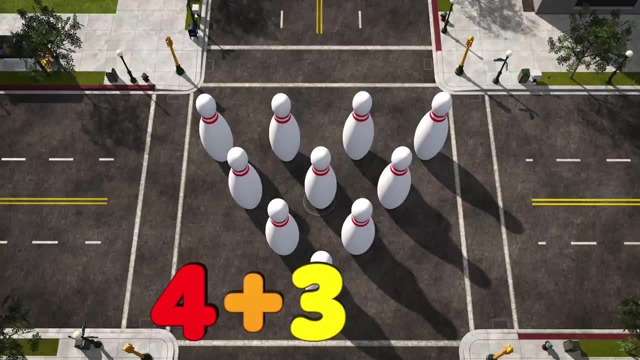 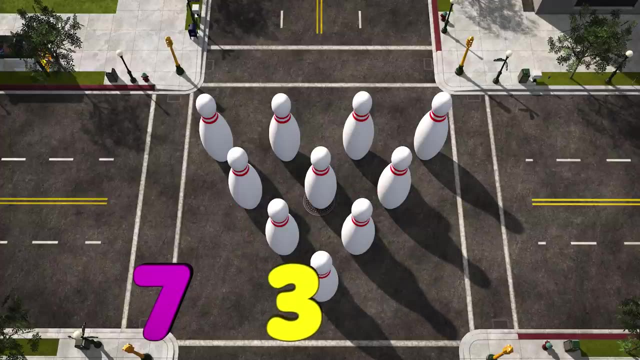 We can use adding. to quickly count them up, This row has four and this row has three, So four plus three equals seven. There are three more, so seven plus three equals ten. There are ten bowling pins set up in the street. 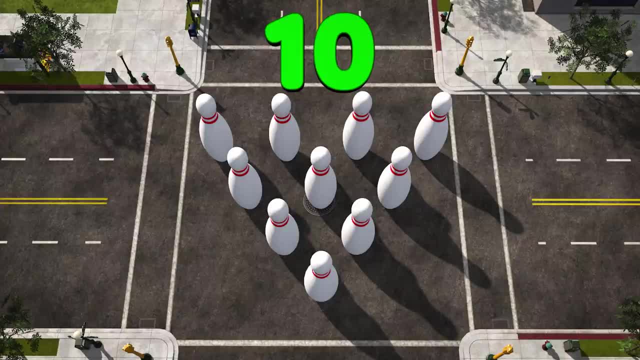 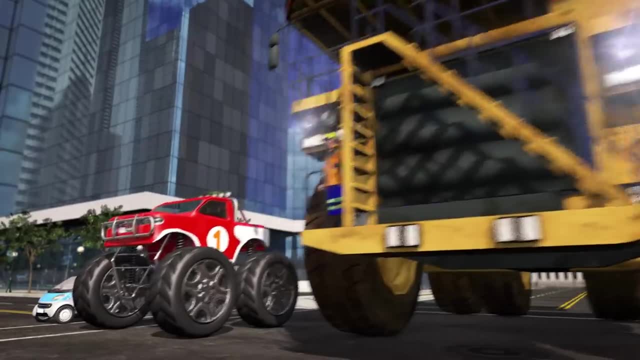 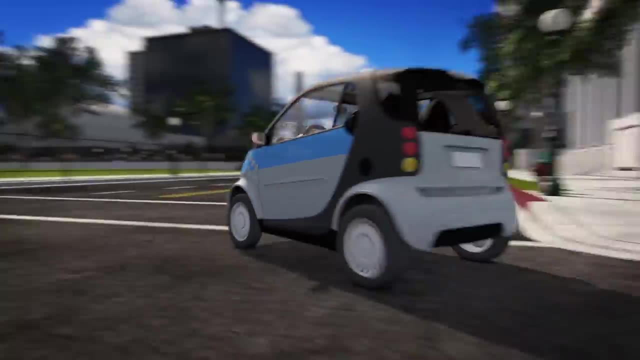 Let's see how many of these pins each vehicle can knock down. Can you guess which one will knock over the most pins? Let's start with the smart car. Okay, little smart car. let's see how many pins you can knock down. Ready Go, little smart car. 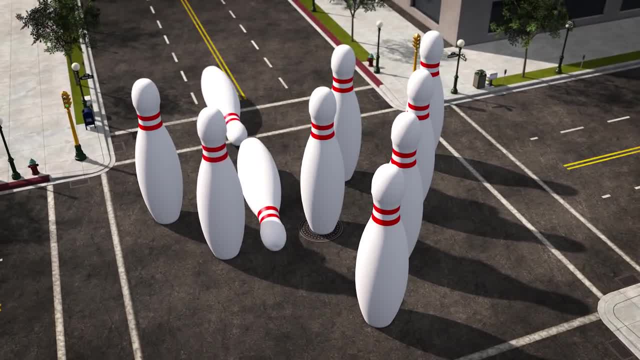 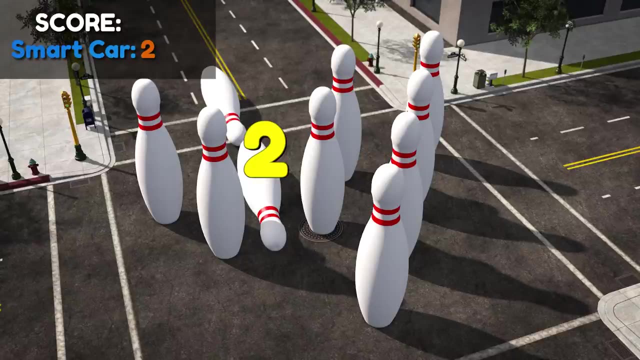 Aw, the little bitty smart car was too small to knock down many of the pins. How many did he get? That's easy, we can just count them One, two. The smart car knocked over two pins. Let's see how many pins the little bulldozer can get. 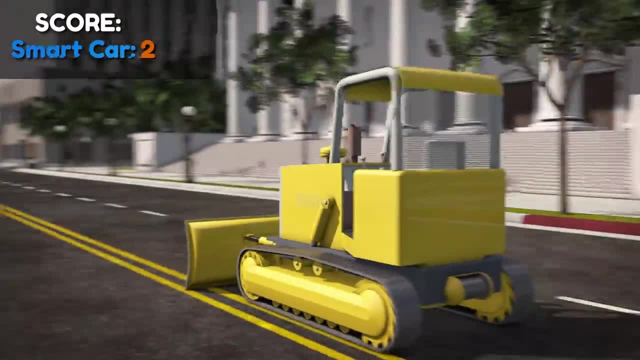 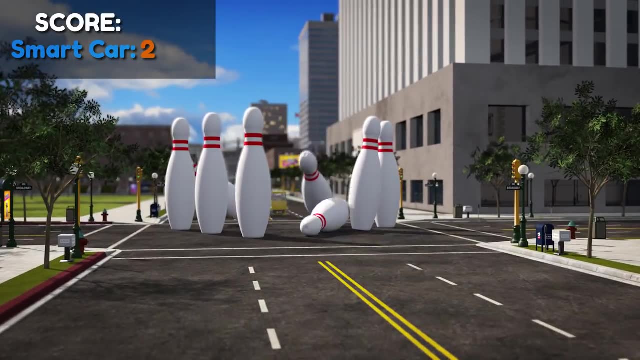 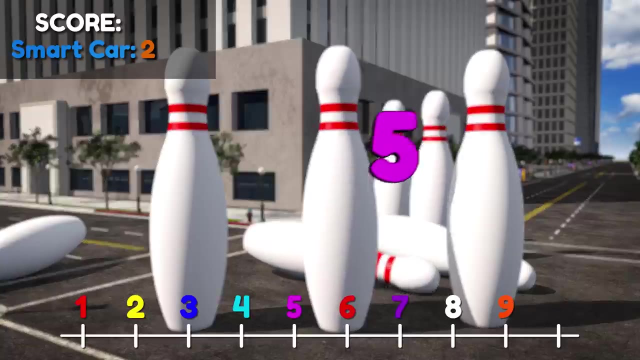 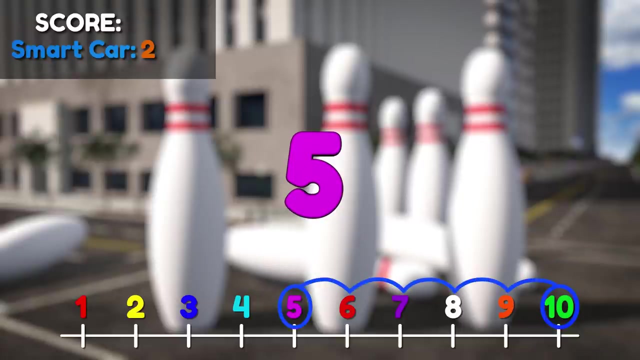 Go little bulldozer. I bet he can knock down more than the little smart car. Not too bad. There are five pins left standing. We know that we started with ten pins, so we can find how many pins were knocked down by subtracting five from ten. 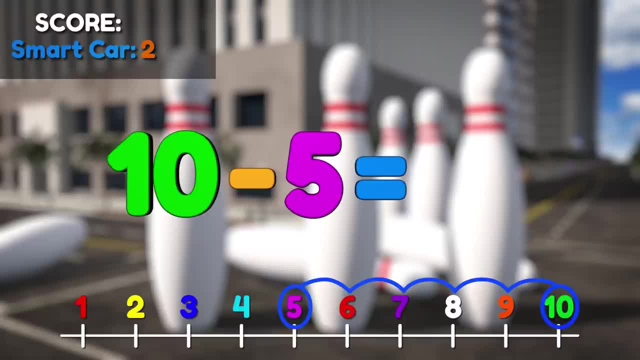 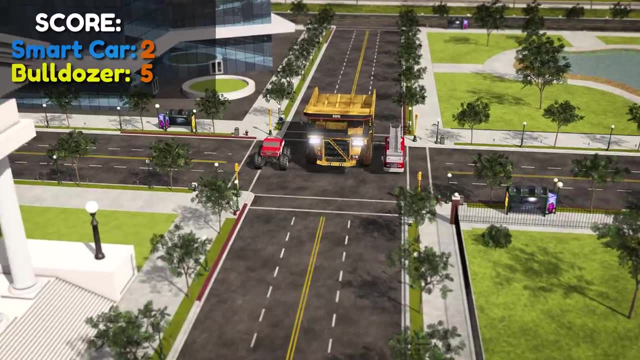 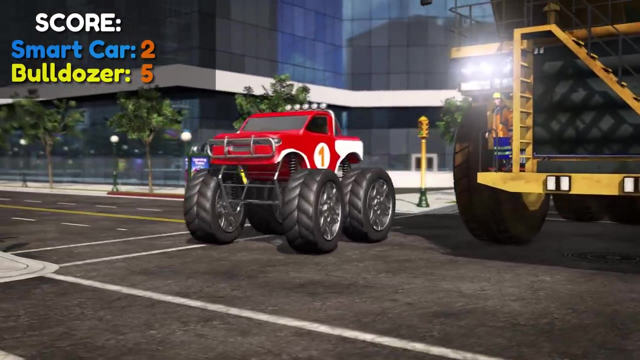 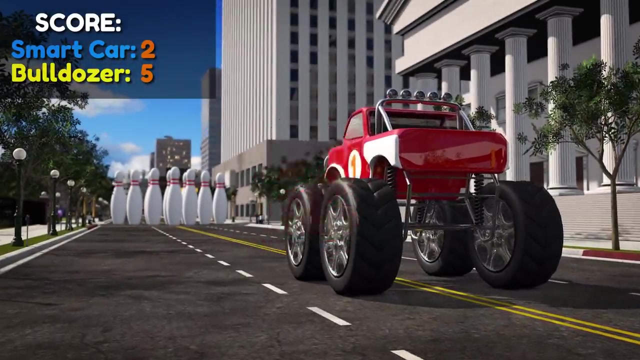 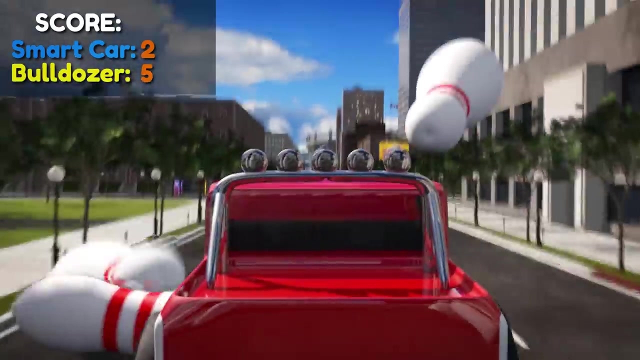 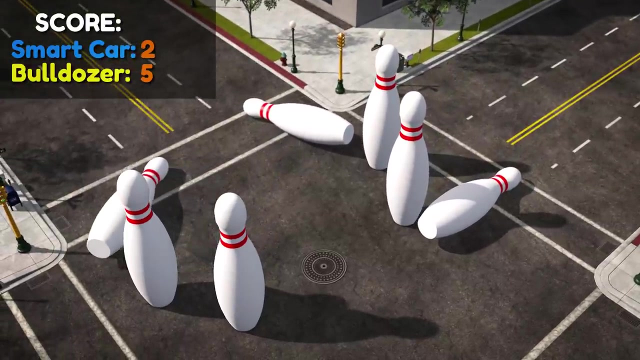 Ten minus five equals five. So the bulldozer knocked over five pins. How many pins do you think the monster truck will knock down? Ready Three, two, one go. Looks like the monster truck knocked down even more pins. There are four pins remaining, so how many did he knock down? 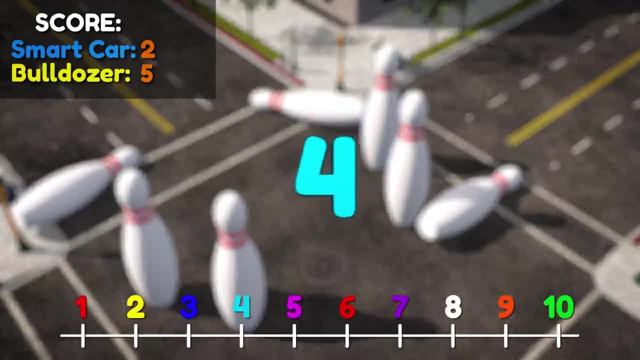 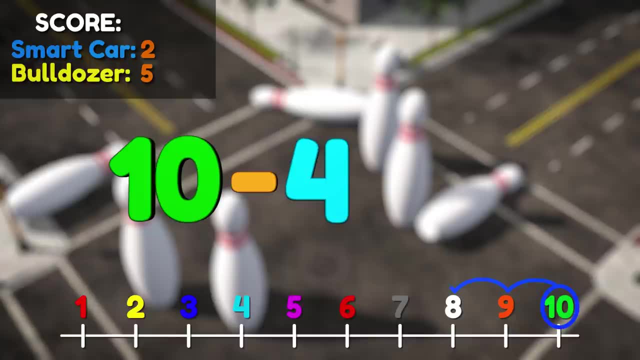 We started with ten pins, So if we subtract the pins that are left, we'll find the number that was knocked down. So ten minus four equals six. The monster truck knocked down six pins. Looks like he's in the lead now. Let's give the fire truck a try.